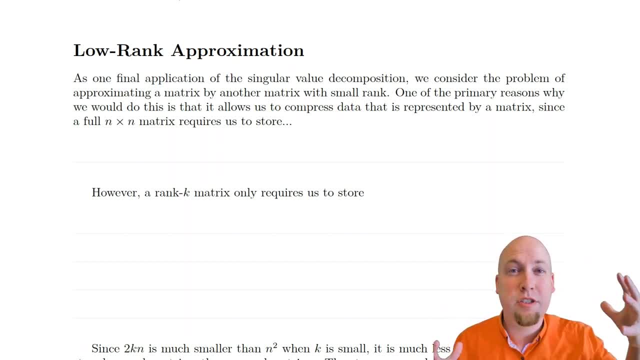 you've got some very, very large matrix and you would like to store this matrix efficiently, More efficiently than just listing out all of the numbers in that matrix. Well, how can you do this? Well, one way is, instead of storing that matrix itself, instead you find some. 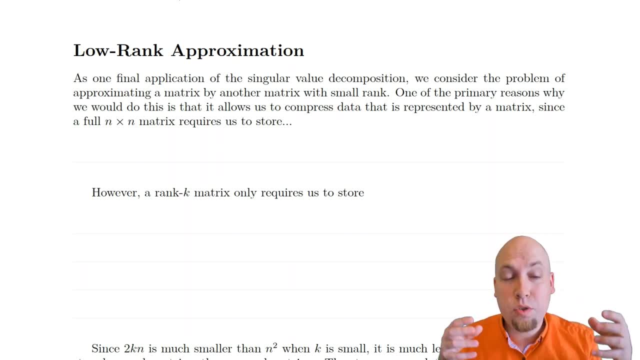 nearby matrix that has lots of structure and store that matrix itself. As long as it's close enough to the matrix you actually care about, maybe that's not a bad thing to do. So that's the idea that we're going to go through in today's lecture And in particular, 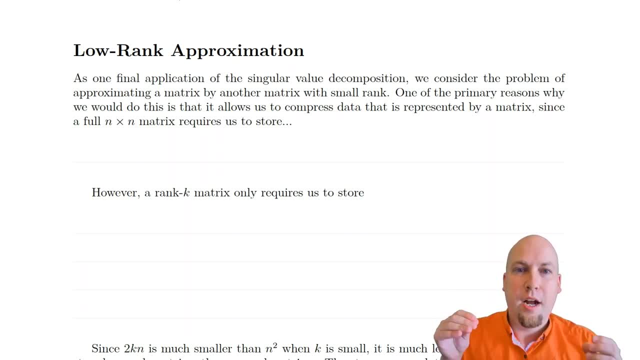 the nearby nicely structured matrices that we're going to find are matrices that have low-rank, And we're going to see that having low-rank makes them easier to store than general high-rank matrices. Okay, so here's the setup. If you want to store, you know, just a general full n by. 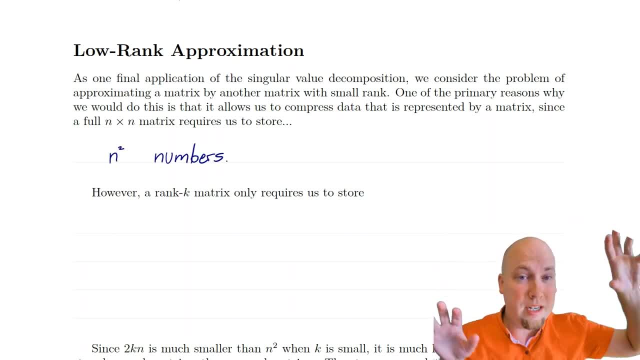 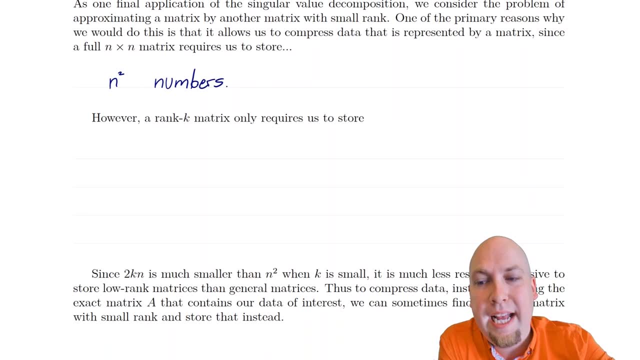 n matrix. you're going to have to store n-squared numbers, right? There are n-squared numbers in that matrix, Okay. Well, instead, if your matrix happened to have low-rank, in particular if it happens to have just rank k, then you could store that matrix via just 2 times k. 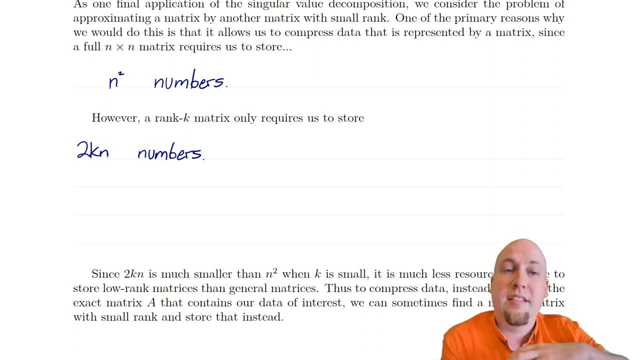 times n numbers. okay, And to see this, let's go back to the singular value decomposition, or actually, even more specifically, the orthogonal rank 1 sum decomposition. Remember, we're going to have to store n-squared numbers, right? You can write every matrix in this. 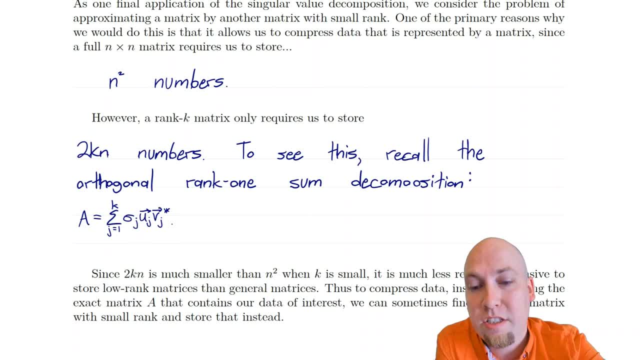 form. If it has rank k, then there's going to be k terms in the sum and it's just going to be singular value times left. singular vector times right. singular vector star. okay, So it turned into a row vector. Okay, And the reason, then, that you can store it in 2 times? 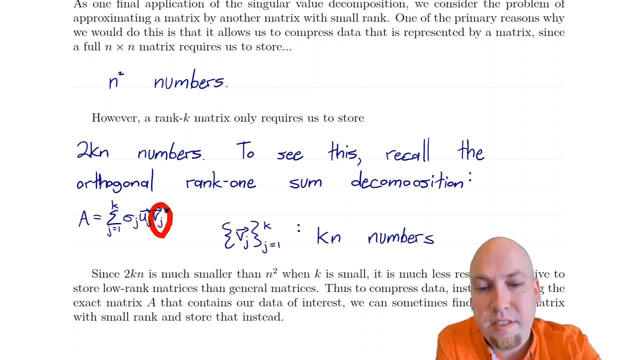 k times n numbers is well, first off, these vj vectors, each vj vector, you can store each one of them via just n numbers, right? Just a vector with n entries And there's k of them. So, overall, k times n numbers to store all of these vj vectors. So you're going. 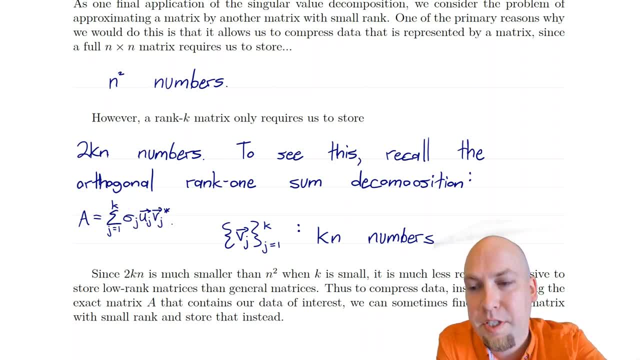 to have n entries And then you can do something similar for these sigma j times uj's. okay, If you just sort of multiply each uj by sigma j and then keep track of these vectors again, each of them has n entries and there's k of these vectors. So overall you're storing. 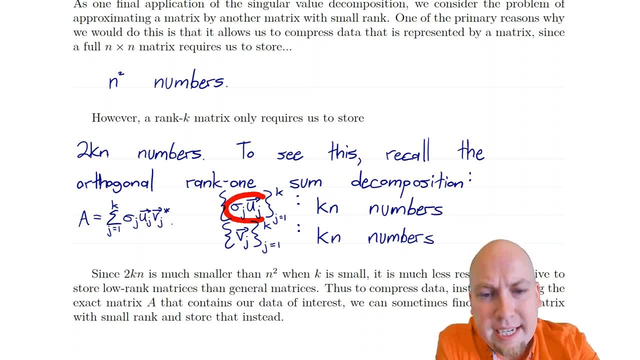 k times n numbers. Okay, The reason that I'm multiplying these guys together is just to make the storage slightly more efficient. You could store the sigmas separately from the uj's, but then you're going to have an extra n numbers that you don't actually need. 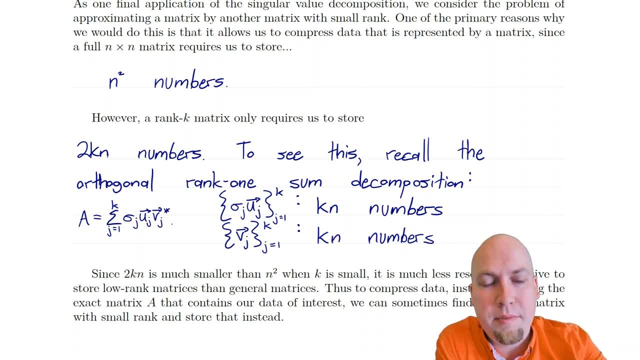 okay, So it's just a slightly more efficient way to do it. if you absorb these sigma, j's Okay. And the point is if the rank of this matrix is small, if k is small, then 2 times k times n, that's much smaller than n squared. So this is a more efficient way of storing. 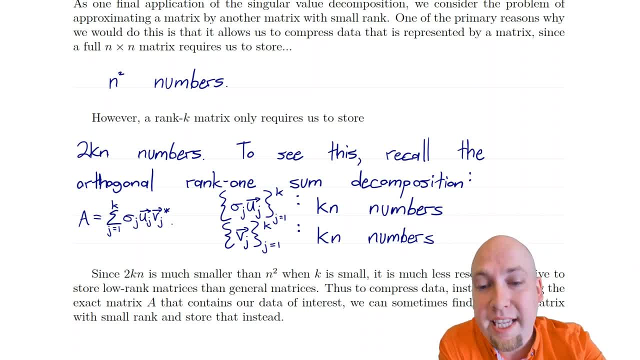 the matrix. Rather than just listing out the entries of the matrix, you list out the entries in this orthogonal rank: 1 sum: decomposition of the matrix. Okay, But I mean not every matrix is going to have small rank. I mean most matrices don't? Most matrices have large. 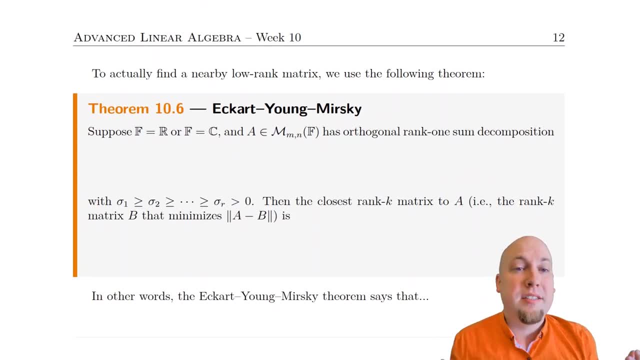 rank, But fortunately there's a theorem that tells us how to find the nearest small rank matrix to any matrix that you start with. Okay, So the setup will be: we start off with our big matrix that we actually care about. Eh shoot. 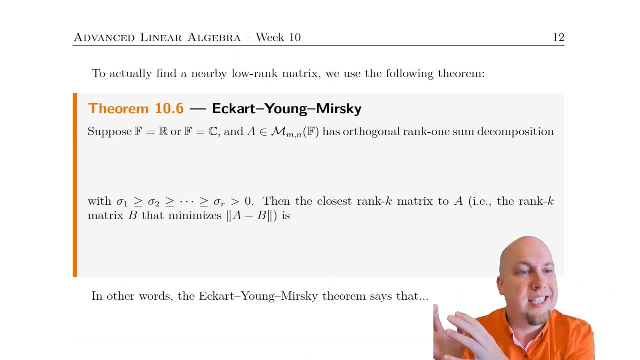 it has high rank, But here's a low rank matrix that's really really close to it. Let's store that guy instead, Okay. So what is the theorem? How do we find this nearby low rank matrix? And here's the setup. Suppose that you've got just some matrix, real or complex entries. 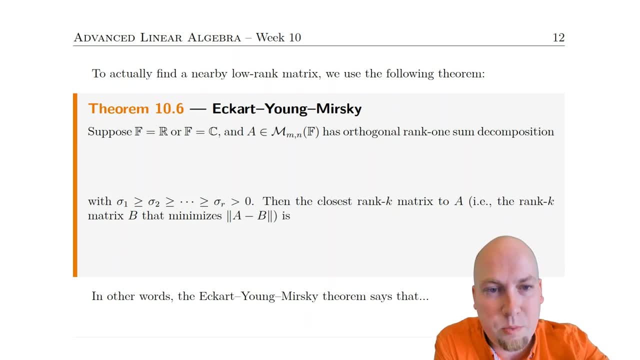 Doesn't actually even have to be square, Okay. So up above, the calculation I did was with square, and you know, m equals n Doesn't have to be that case, It can be rectangular as well. Okay, And then? well, what we're? 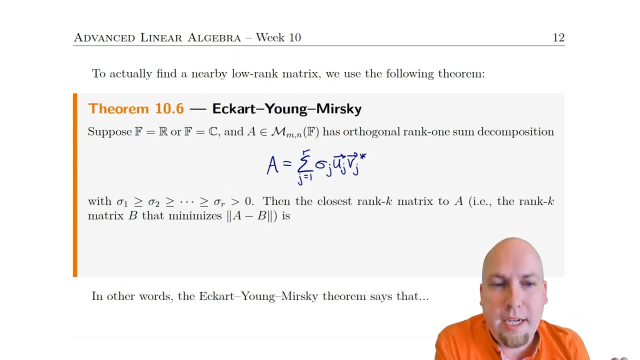 going to do is we start off with some orthogonal rank 1 sum decomposition of our matrix? Okay, And then what you do to find the closest rank k matrix to that matrix? this matrix has rank r, Okay, And r might be very large, I don't know. Okay, It's just. whatever the rank of. 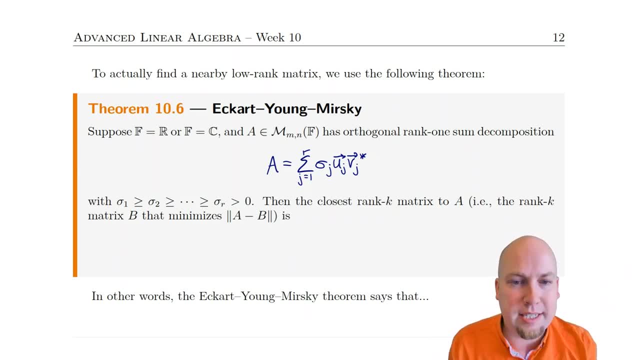 a is. But then to find the closest rank k matrix to a, all you do is you take this orthogonal rank 1 sum decomposition and you truncate it. Okay, You just take the first k matrix, you put it away from the nearest k. you put it away from the nearest k matrix and you change. 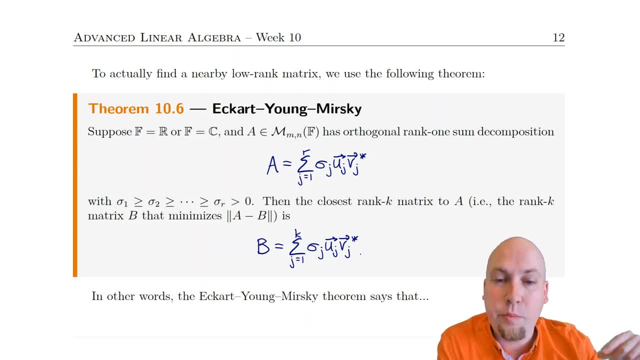 values. I think, uh, a product, and it's kind of odd. So a product and I say this is A product and I say this is A product, a product and I say this is a business unit for that particular identity. Okay, So possibly a product, a product where given nothing and nothing takes. 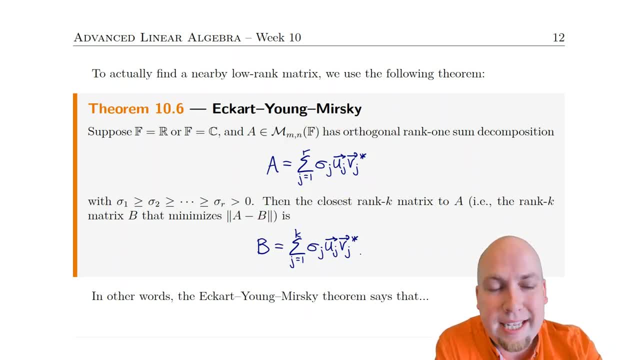 any place, And you could even visualize an exp孩子 simply moving around a local array. Okay, This is the horizontal rank 1 sum decomposition And it's the exact same as this one, except you're just taking the k largest terms. You're taking the k terms. 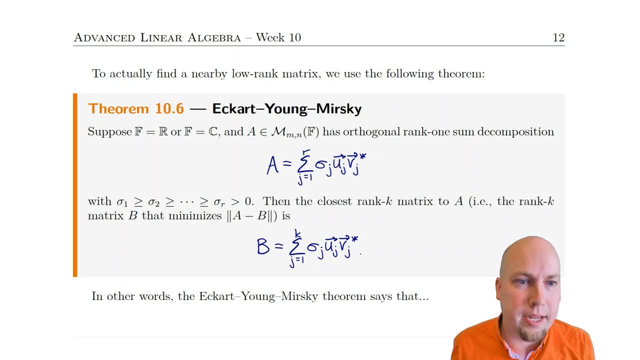 corresponding to the k largest singular values of a, and then you're throwing away all of the terms corresponding to the small singular values of a. Okay, So in other words, what's okay if I keep missing bulk from Сchanca上 paS All the terms that go with both the 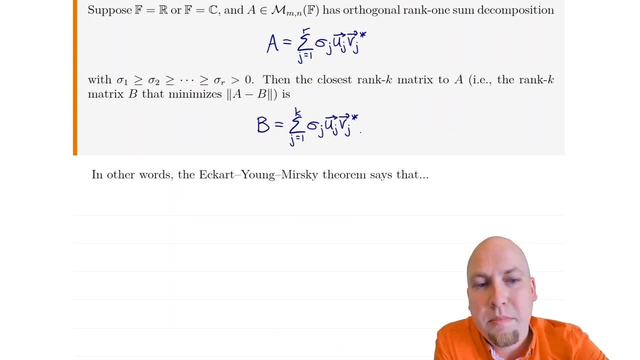 one way of looking at this theorem is this Eckert-Young-Mersky theorem, the theorem we just went through. One way of looking at it is: it's saying that the singular value decomposition, or equivalently this orthogonal rank 1, sum decomposition, it organizes the matrix into 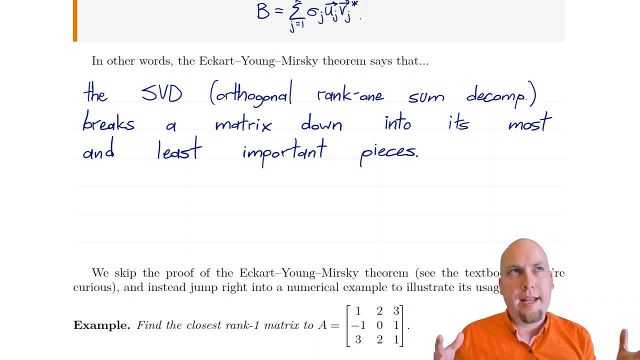 its most and least important pieces. Sort of it's saying that you know, sigma 1 times u1 times v1 star, that's like the most important rank. 1 piece of A Okay, and then sigma 2 times u2 times v2. 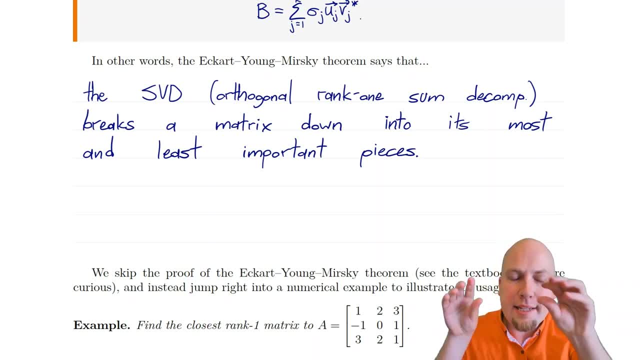 star. that's the second most important rank 1 piece of A and so on down the line all the way down to you know, some of the singular values are zero and those pieces are very not important. they're just zero matrices. Okay, so it sort of creates a hierarchy of: yeah, this is a very 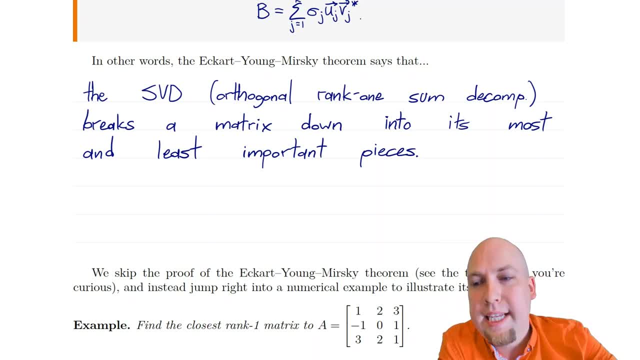 important piece of A, this is the next most important piece of A, and so on down the line. And to create these rank k approximations you just take the k most important pieces, okay, Or maybe another way of phrasing this: the large singular values of a matrix. they provide sort. 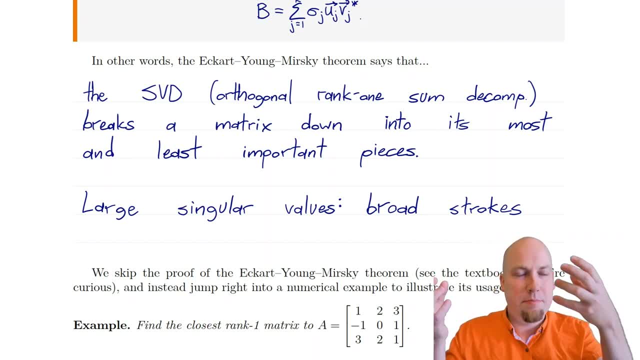 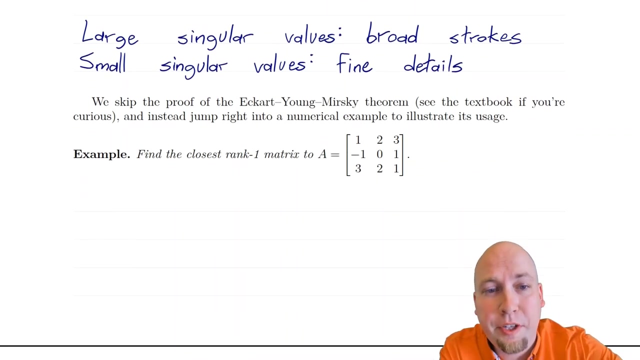 of the broad structure. Okay, so we're not going to prove this theorem. The proof is in the textbook, if you're curious. Instead, we're going to jump right into a numerical example here. So what we're going to do is we're. 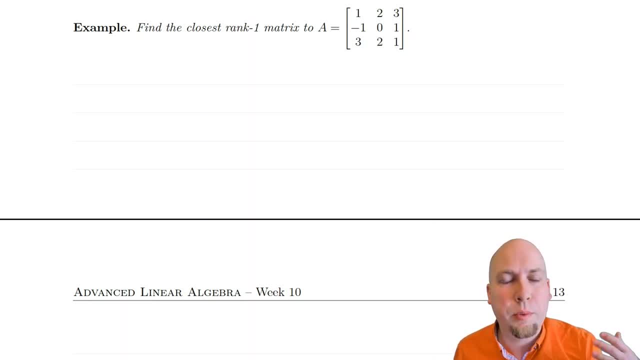 going to use this matrix. you know 1,, 2, 3, minus 1, 0, 1, 3, 2, 1.. We've seen this matrix a couple times, So the reason I'm using this particular matrix is because we've already. 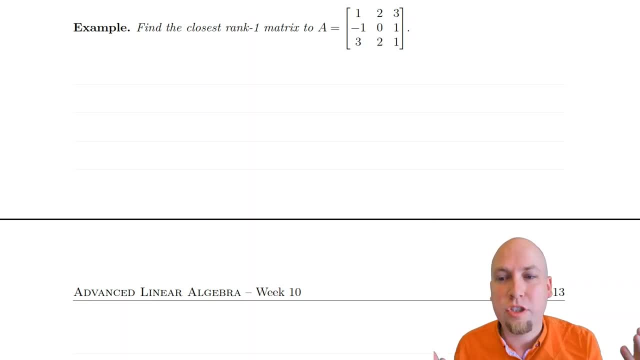 computed a singular value decomposition of this matrix, so we can just leech off of it. Okay, we computed a singular value decomposition of this matrix back in lecture 34, when we first learned about the singular value decomposition. and here it is. This is what we 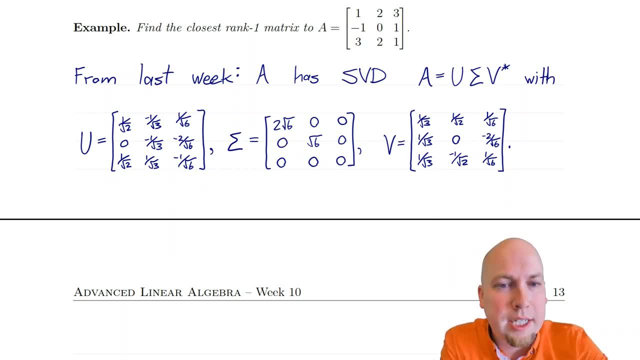 computed. So the matrix, the unitary matrix u on the left is there, and then the diagonal matrix sigma in the middle is there and the unitary matrix v on the right is there. Okay, so we're going to. So the way that we compute the closest rank 1 matrix based on the singular value, decomposition. 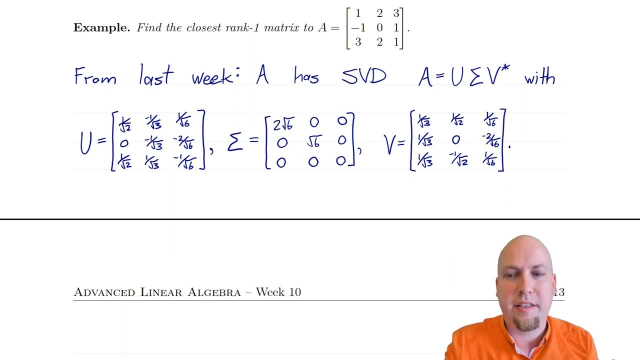 is well remember how the singular value decomposition is related to the orthogonal rank 1 sum decomposition. What you do is you just give names to the columns of u and v, right? So the first column of u is u1,, second column of u is u2, third column is u3, and similarly for v. 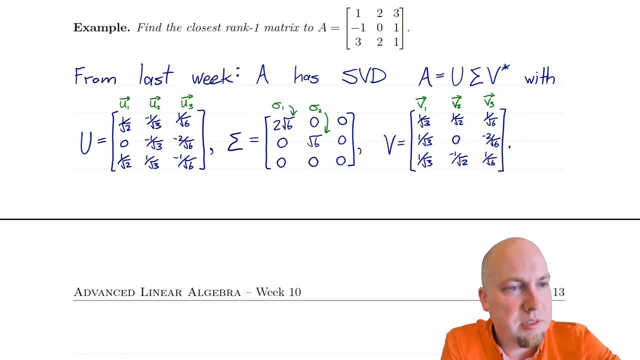 First column is v1,, second column is v2,, third column is v3, and then sigma 1 is the first singular value and sigma 2 is the second singular value, the diagonal entries of sigma. okay, And then you just throw all of these pieces into the formula described by the Eckert-Young-Mersky. 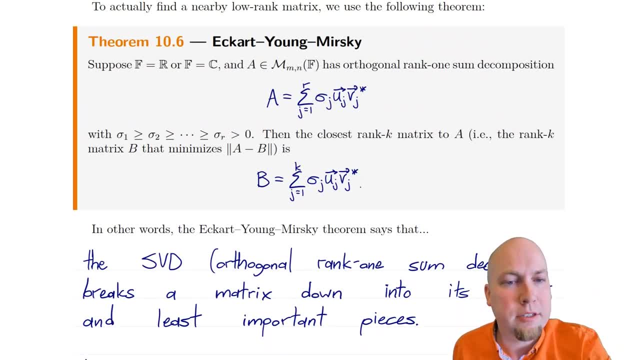 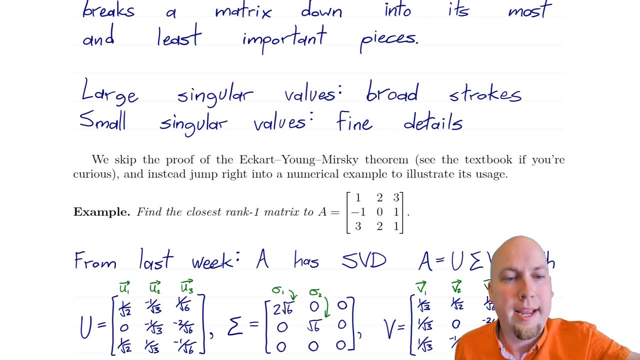 theorem okay. So because we want the closest rank, 1 matrix. you know it's a sum with just one term, so we forget about the sum, It's just sigma, 1 times u1 times v1, star, okay, And that'll. 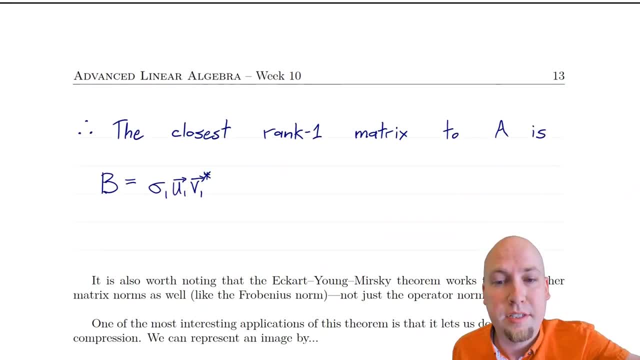 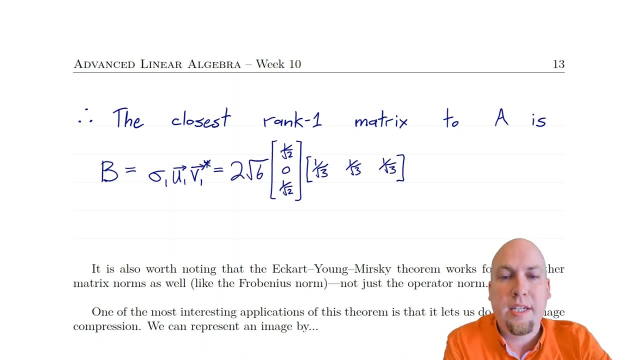 be the closest rank 1 matrix to A. okay, So the closest rank 1 matrix to A, it's just sigma 1 times u1 times v1 star. okay, And we just plug those in. okay, What is sigma 1?? Ah, we just saw. 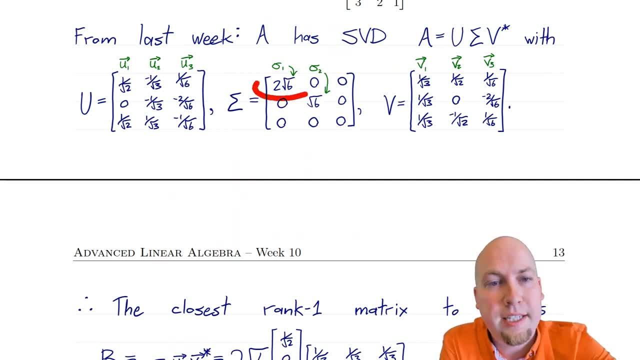 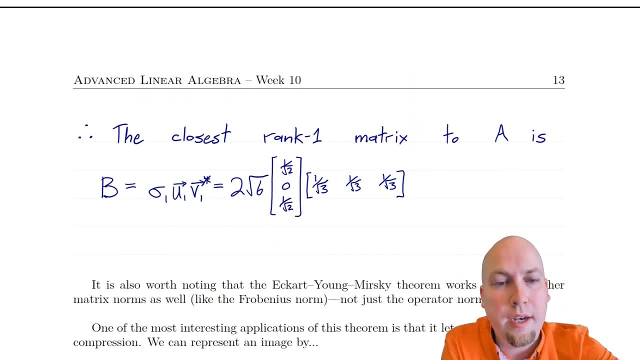 root 6, right, It's that first diagonal entry right here. And then what's u1?? Ah well, it's this column vector here, so we just plop that down here. Here's u1.. And then what's v1 star, Well, 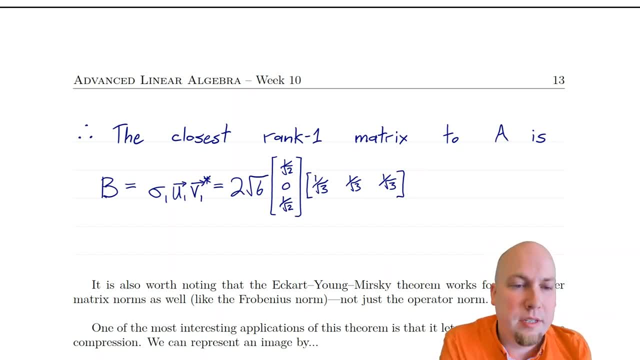 we take the first column of v and we conjugate, transpose it. okay, So now it's a row vector And then you just do matrix multiplication: multiply all those things together and fortunately, all the square roots cancel out and it becomes very nice. You just get this matrix. 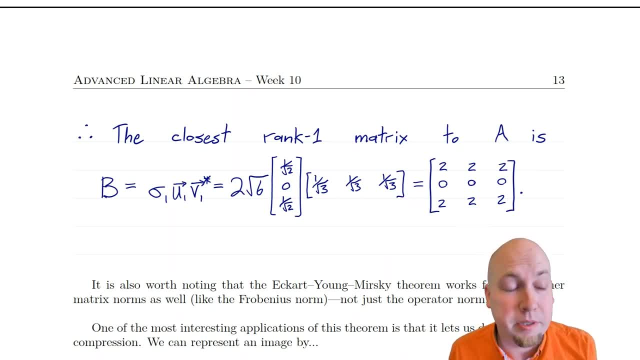 2, 2, 2 in the first row, 0, 0, 0 in the second row and 2, 2, 2 in the third row. okay, So straightforward to check that if you want to convince yourself that that is a rank 1 matrix. 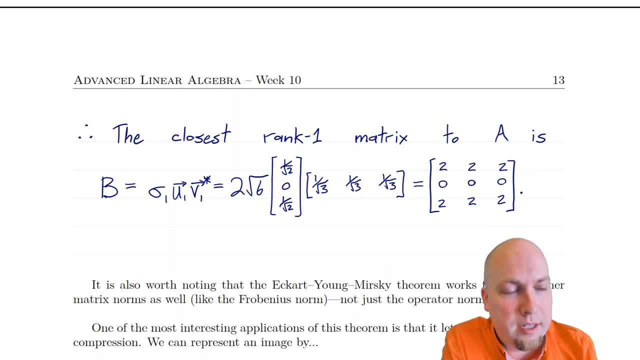 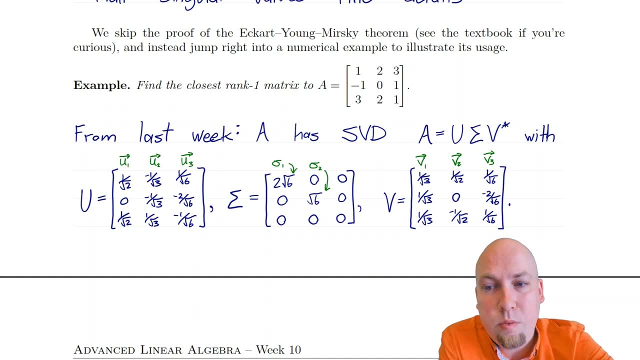 yeah, it is okay, You do your row operations. you're just going to get one non-zero row, But it's actually the closest rank 1 matrix to this original matrix that we started with. out of all the rank 1 matrices out there, it is the one such that A minus B has smallest operator. 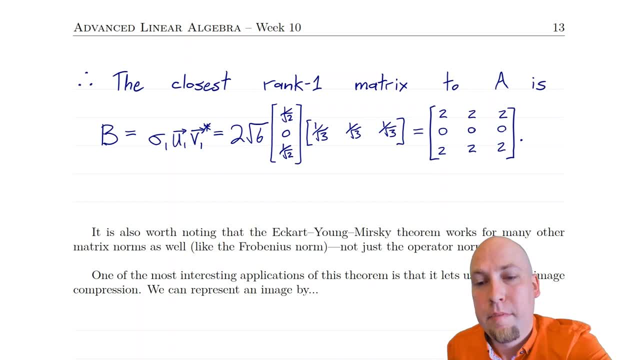 norm. okay, And maybe just as a little side note here, it's worth noting that I mean because of the orthogonal rank 1 sum decomposition, if I were to add sigma 2 u2 times v2, v2 star to B. 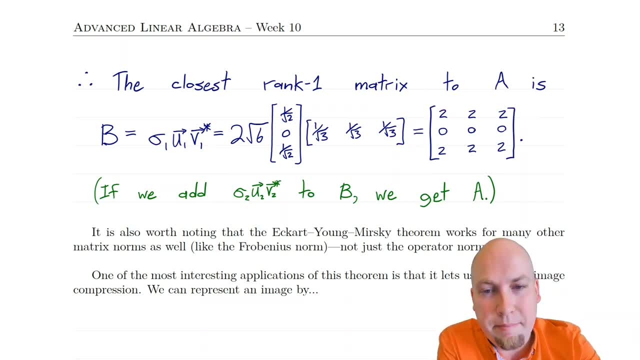 to this matrix. here we would get exactly A right, Because I mean the orthogonal rank 1 sum, decomposition of A itself. it's just this term plus this term, right, It's a rank 2 matrix, so it just has these two terms in it. And to get this matrix B, all we did was we forgot about the. 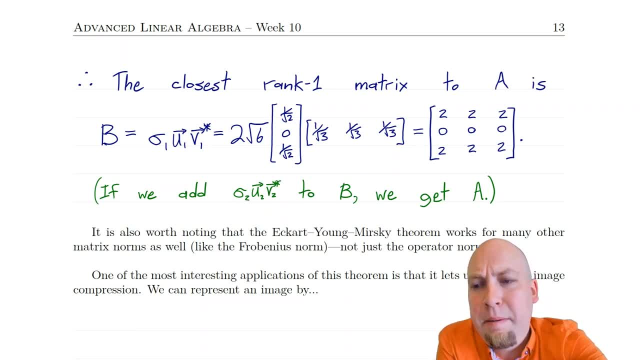 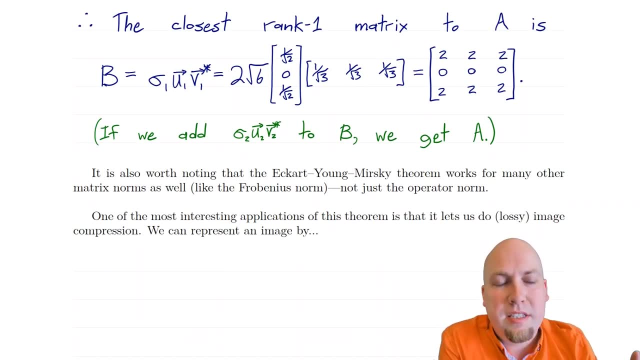 second term. okay, And as maybe one more note before we go on to a certain nice application of this theorem. this theorem is a little bit more complicated than the first one, but it's this Eckart-Young-Mersky theorem, this approximation theorem, it works, the exact. 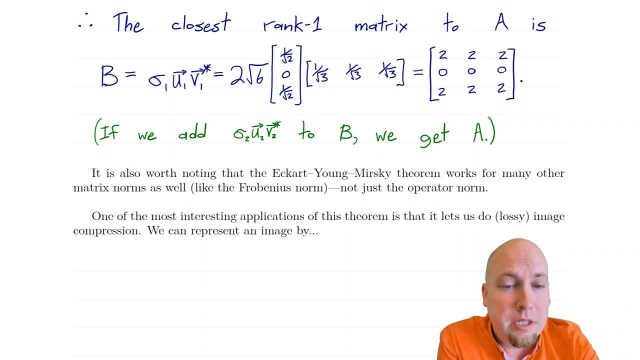 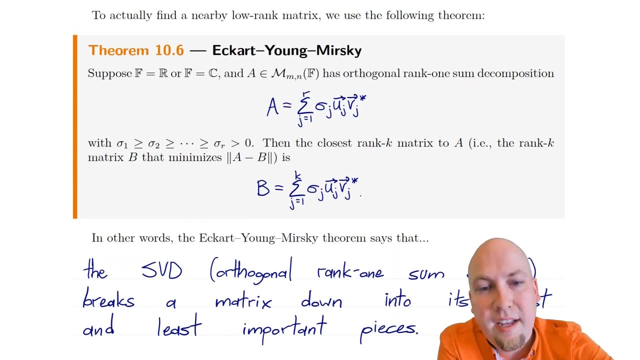 same with lots of other matrix norms. For example, it works the exact same with the Frobenius norm. So if you don't like the operator norm here, if you don't like measuring the distance between matrices via the operator norm, then you can measure it via the Frobenius norm as well. 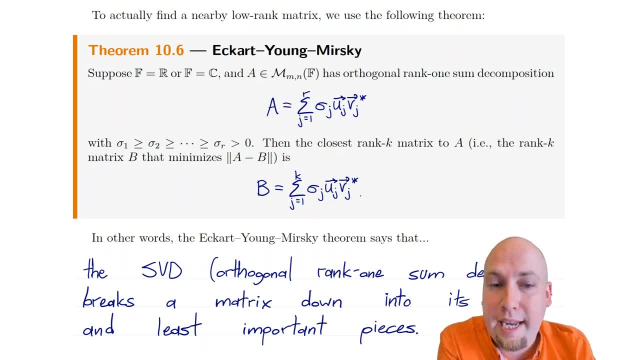 and the conclusion is the exact same. This is still the closest rank K matrix, And this is true even for lots of other norms, For any matrix norm that is what we call unitarily invariant- okay, So any matrix norm that has the property that it is unchanged under left or right multiplication. 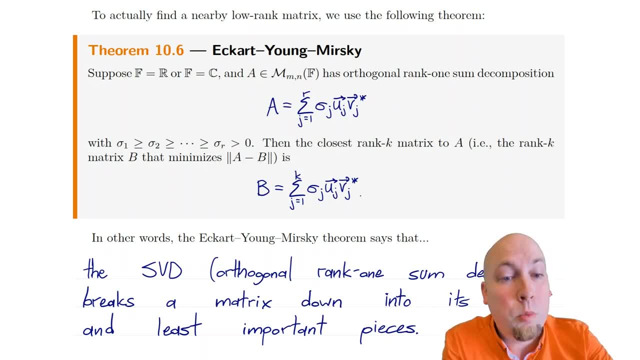 by a unitary matrix. any matrix with that property will satisfy this theorem. So you can throw in that matrix norm there and the conclusion will still be: this is the closest rank K matrix. Okay, so if you don't like the operator norm for whatever reason, that's okay. 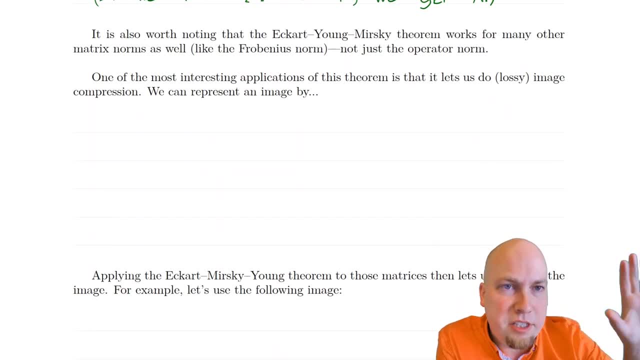 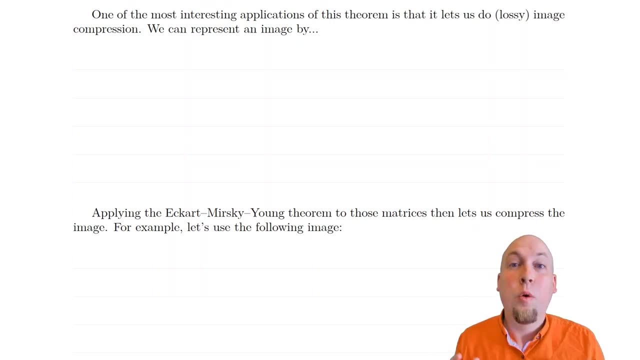 Use some other norm, As long as you choose it to be unitarily invariant, the same conclusion will still hold. You can still use this theorem to find the closest rank K matrix. One of the really neat things we can do with this theorem is we can do image compression with it. okay, But before we can, 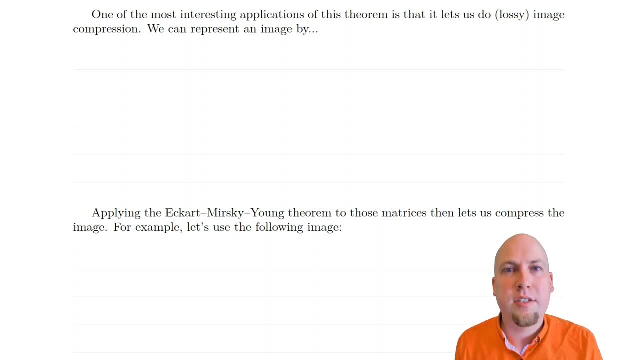 do that? we need some way of representing an image via a matrix or matrices, And one of the simplest ways to do this is to represent an image via three matrices. okay, So we're going to use one matrix to describe how much red there is in each pixel of the image, one matrix to represent how 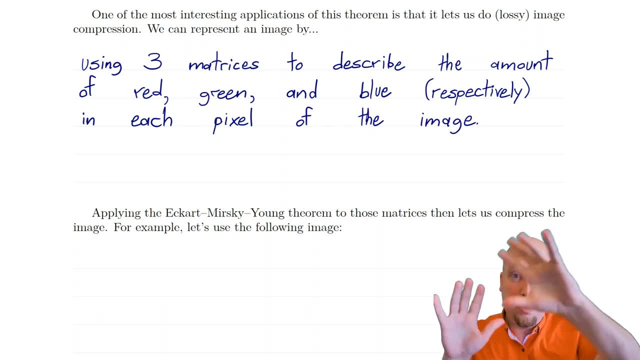 much green there is in each pixel of the image and one matrix to represent how much blue there is in each pixel of the image. okay, And then if we use an additive color scheme, then well, every single color can be written as some amount of red plus some amount of green. 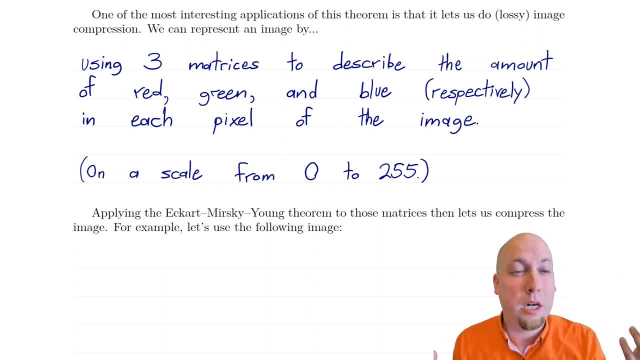 plus some amount of blue. okay, Those are our three primary colors, So we can describe arbitrary colors in this way then. okay, And in particular, we're going to use a scale from 0 to 255, but that's sort of an implementation detail, that's not particularly important. So 0 is going. 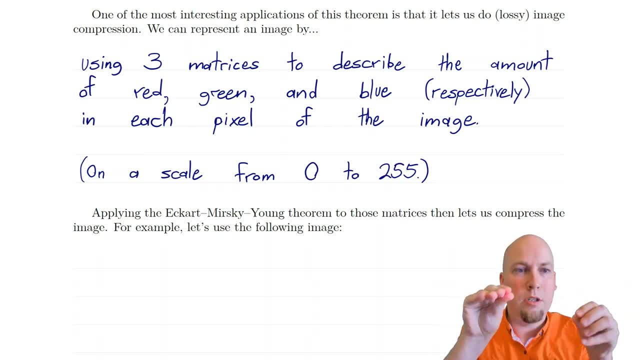 to mean there's none of that color, There's no red or no green or no blue. And 255 means there's tons of it, like it's all red or it's all green, it's all blue. It has the maximum amount of that. 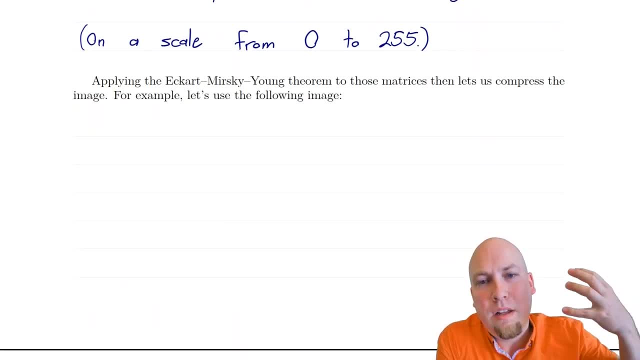 color that you could have, okay. So if we use the Eckhart-Mersky-Young theorem applied to these three matrices, then what's going to happen is we're going to find nearby matrices that have low rank and they're going to generate images that look a lot like the original image but are 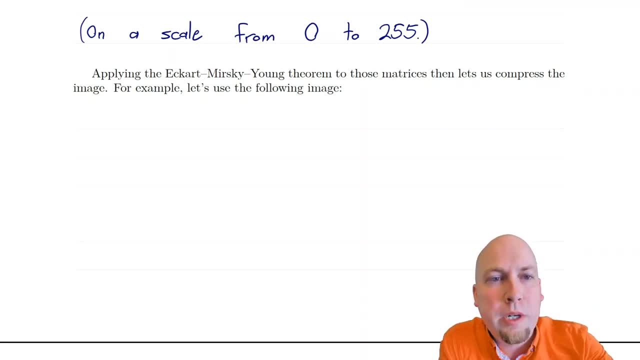 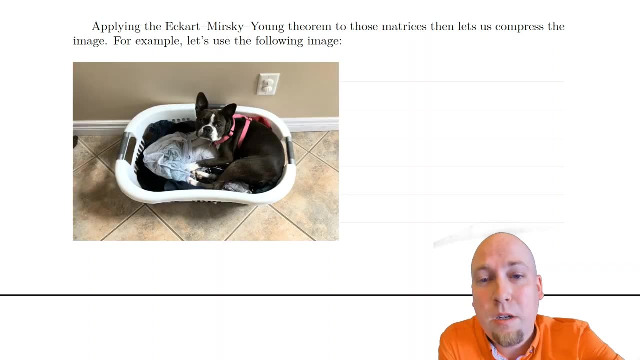 much easier to store. you know We're going to be able to store them using fewer real numbers than the original matrices that we started off with. Okay, so let's illustrate how this method works via an example. okay, So I'm going to do image compression on this image here. okay, So? 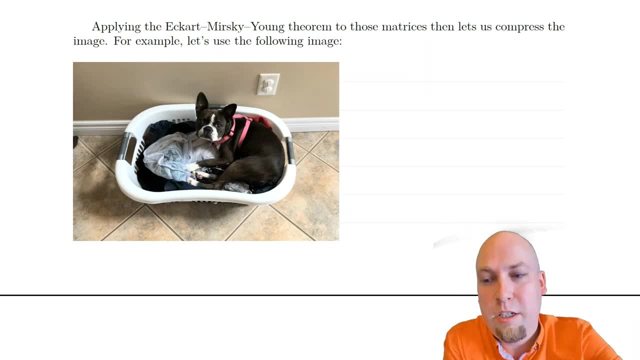 this is my seven-month-old puppy, Maisie. She's been very bad. She's gotten into the laundry basket. So bad, Maisie, And her punishment is going to be: I'm going to compress her. okay, I'm going to take this image and I'm going to reduce its rank and see what happens to the resulting. 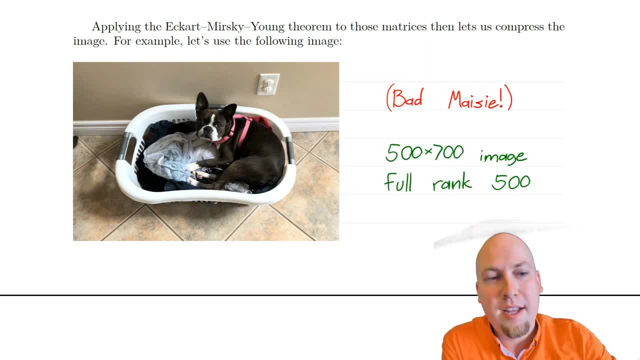 image when we do that, okay. So to start off with this photo here. it's a 500 by 700 image. okay, It has 500 pixels if you count top to bottom and 700 pixels if you count left to right, And it 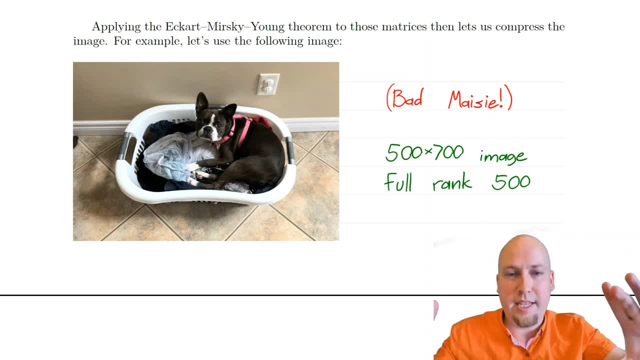 has full rank 500,. okay, So each of the three matrices that I used to represent this image, they have full rank 500, which is as large as could possibly be because they're 500 by 700 matrices. okay, But if I do compression to these matrices via the Eckert-Young-Mersky, 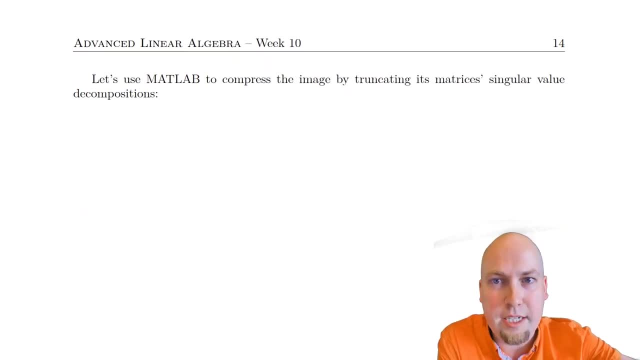 theorem. so I have MATLAB code that did this for me. I compute the singular value decompositions of these three matrices and then I just truncate them and then multiply things back together. I'm going to get lower rank matrices that are similar to the original matrices and therefore 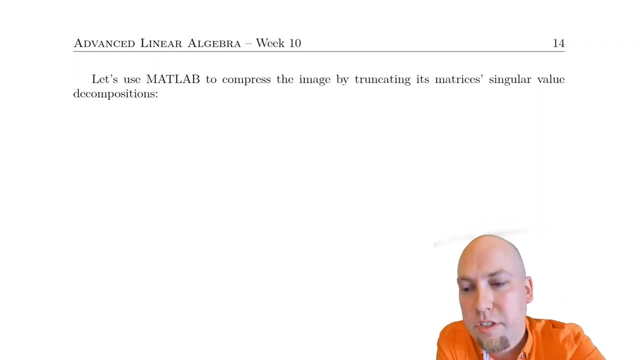 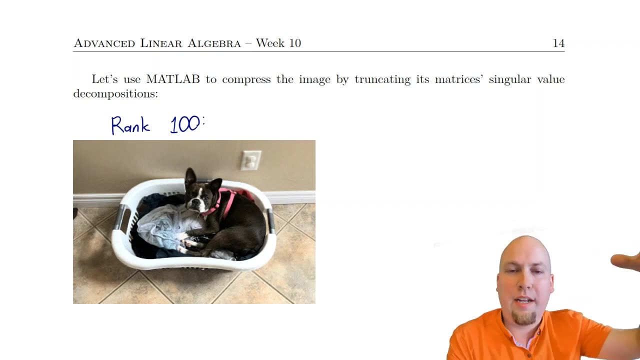 lower rank images that are similar to the original image. So to start off with, let's do a rank 100 approximation of this image. So remember it started off as rank 500. So what I've done now is I've taken that 500 term, rank one, orthogonal sum decomposition, and I've deleted 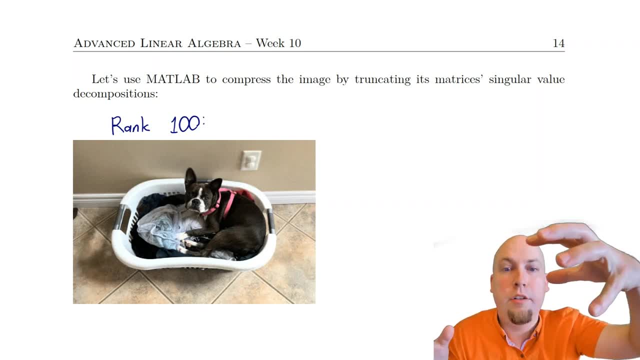 400 of the terms in that sum, and I've left only 100 terms in that sum. okay, So this: this is what the image looks like if we represent via rank 100 matrices using the Eckert-Young-Mersky theorem. 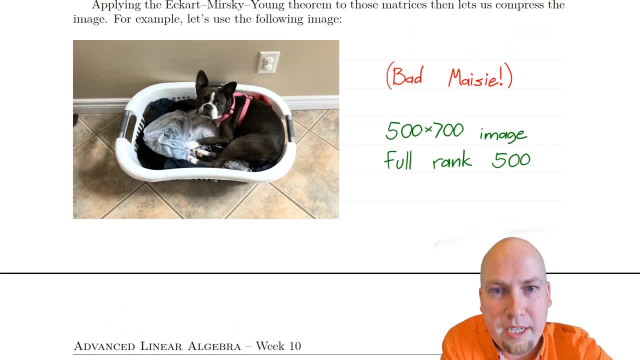 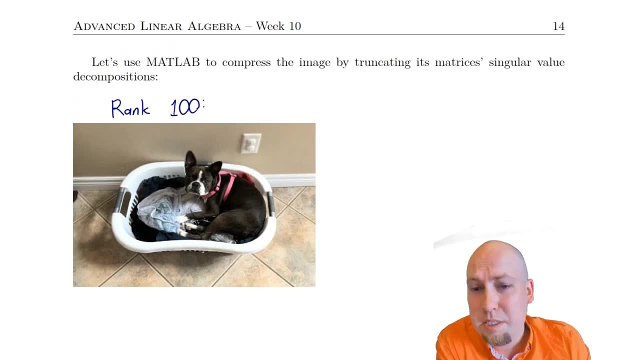 okay, And I'm going to scroll back up to the original image just for comparison. It's pretty good, right? I mean, that's the original image. If we truncate down to just 20% of the singular values, it still looks pretty good Like. if you look closely, you'll see that the original image is. 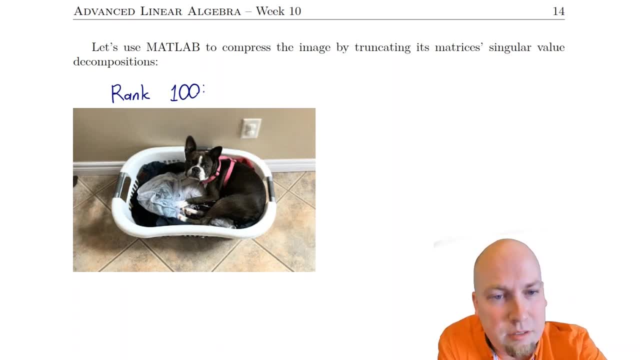 especially on some of these flat spots you can see it doesn't really look as flat as it should Like. there's some graininesses and stuff like that, But overall it's pretty good. Like you certainly get the shape of the image. You get most of the image just by using those 100 out of 500. 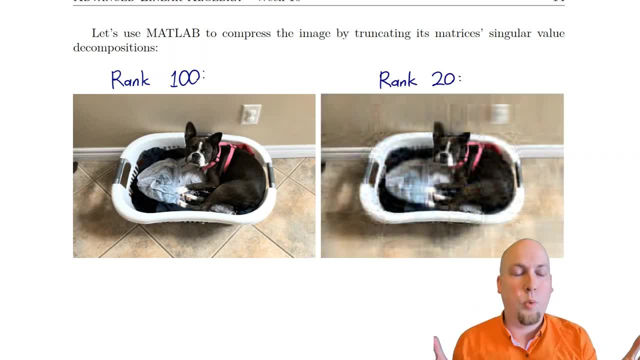 singular values If we go down, even lower down, to rank 20, so now we're only using 20 out of 500 singular values. now it gets a lot worse right Now. now you can see that it's noticeably grainy. 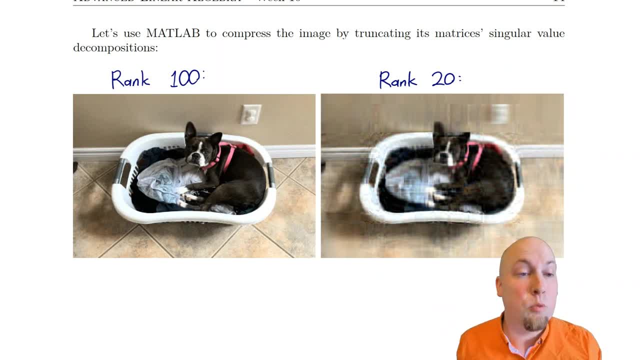 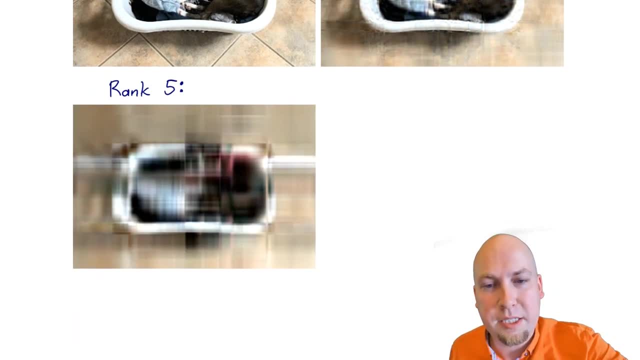 This is what the image looks like as just represented via rank 20 matrices, And we'll go a little bit further just for the sake of illustration. If you go down to rank 5, well, you can see it's pretty atrocious now, but you're only using 5 out of 500 singular values. So I 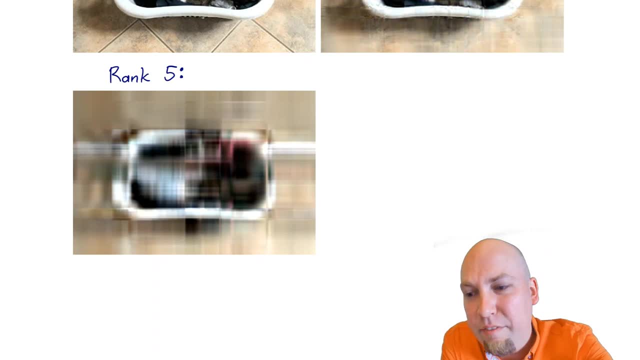 mean we kind of expect that it's pretty atrocious. okay, But even just using 1% of the singular values- like you at least get sort of the color shape of the image right. You can see that there's sort of a white border around here with something darker on the inside- the dog and something. 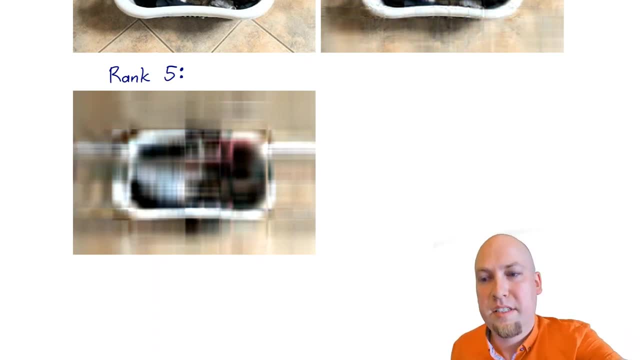 lighter on the outside, the wall and floor. okay, So you still get sort of the color shape of the image. okay, So I'm going to go down to rank 5, and I'm going to go down to rank 5, and I'm going to go down to 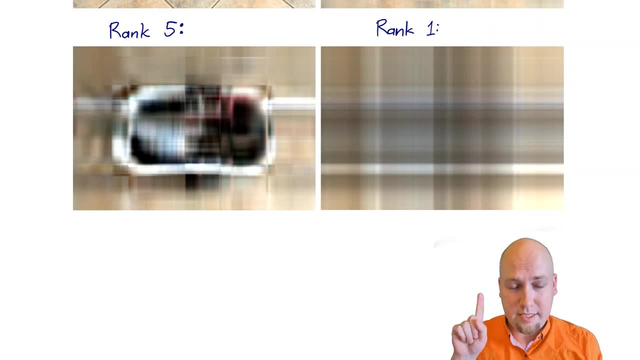 rank 1, then something really interesting happens. actually, okay, So this is just using 1 of those 500 terms. I mean, of course, it's a terrible approximation. okay, You're using 1 of the 500 terms from the original sum in this matrix, But something really neat happens here.